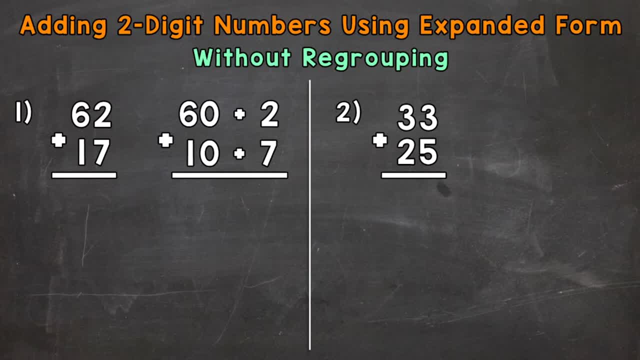 really helps give us a deeper understanding of addition. So let's jump into number one, where we have 62 plus 17, and the first thing we want to do is put both these numbers into expanded form. I've already done that to the right. So for the 62, the 6 has a value of 60. It's in the tens place. 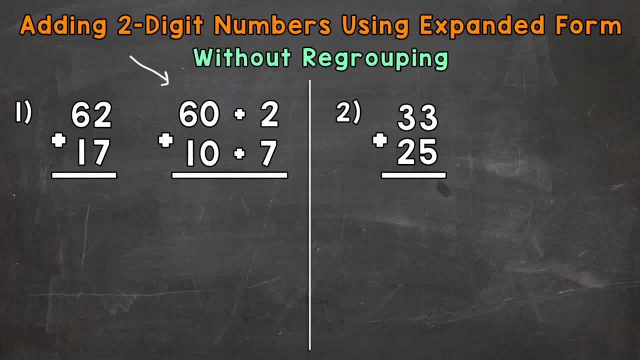 so it represents six groups of 10, therefore has a value of 60.. The 2 is in the ones place, so it represents two ones and has a value of 2.. Now, as far as the 17 goes, the 1 in the tens place represents one 10 and has a value of 10.. 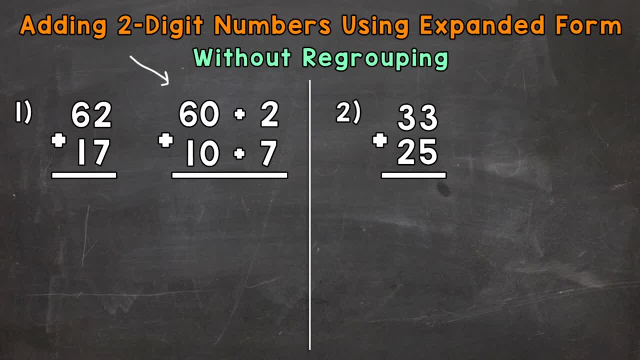 The 7 is in the ones, so that represents seven ones and has a value of 7.. Notice how the ones are lined up right here, and then the tens are lined up right here. Now we're ready to add. So 2 plus 7 gives us 9.. Two ones plus seven ones gives us 9 ones. 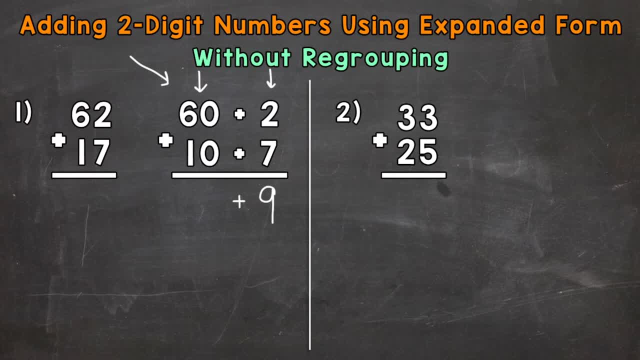 Bring down our addition sign and now we add the tens. So 60 plus 10 gives us 70.. Always add the ones first and then the tens. Now let's add our 70 and the 9. So the tens and the ones. 70 plus 9 gives us an answer of 79.. 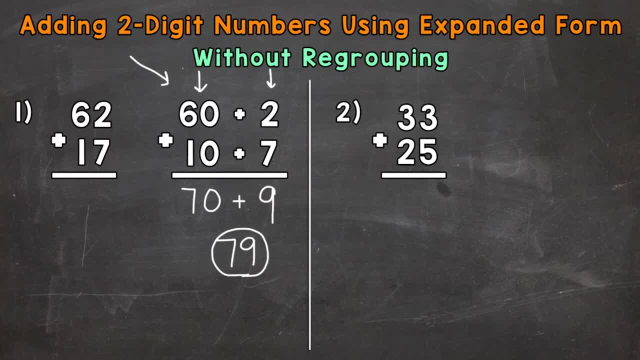 Let's go over to the left at the original problem and add the inside one. Let's go to the left at the original problem and add the inside one vertically, so straight up and down, and see if we get the same thing. so we do the ones first. 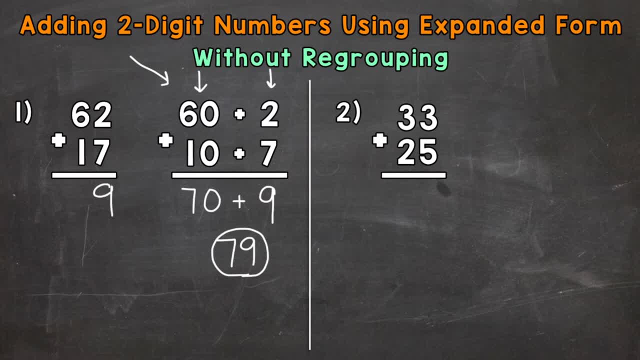 two plus seven is nine, and then we do six plus one, which is seven. we are actually doing 60 plus 10, because that six and that one, those are in the tens place and from our expanded form we understand that that is 60 and 10 and it gives us a seven in the tens place which has a value of 70. 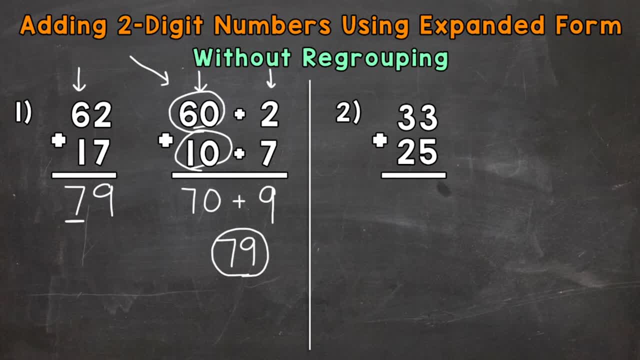 so that expanded form really breaks down the problem and, like i said before, gives us a deeper understanding of addition. so either way we do it, we get 79. let's move on to number two, where we have 33 plus 25. so the first thing we need to do put both of these in expanded form. 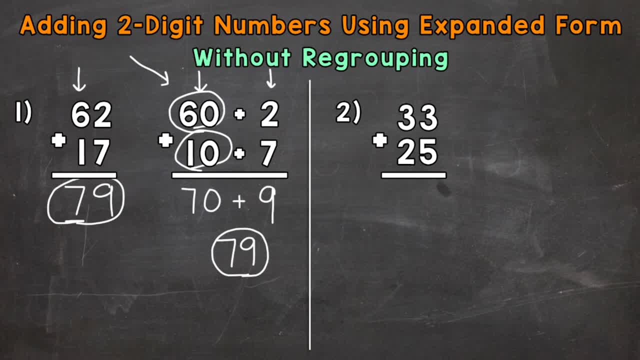 let's do the 33 first. so the three in the tens place has a value of 30. it represents three groups of 10, so 30, plus the three in the ones has a value of 3 because it's representing three ones, so 30. 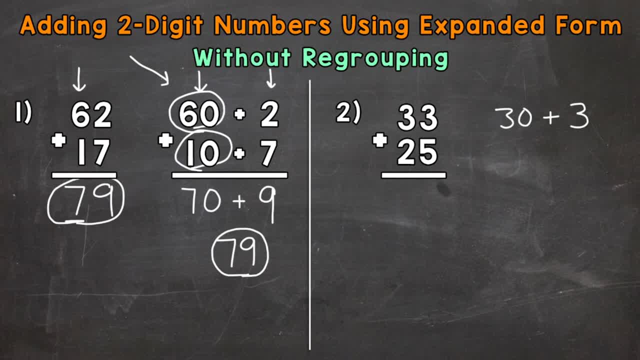 plus 3. now let's do the expanded form for 25. the two in the tens place has a value of 20 plus the five. so that's the first thing we need to do: put both of these in the tens place. and from our expanded form let's move on to number two. so the first thing we need to do, put both of these in the tens. place has a value of 30. so the three in the tens place has a value of 45 and the ones has a value of 40. so that's the first thing we need to do: put both of these in the tens place has a value of 45 and the ones has a value of. 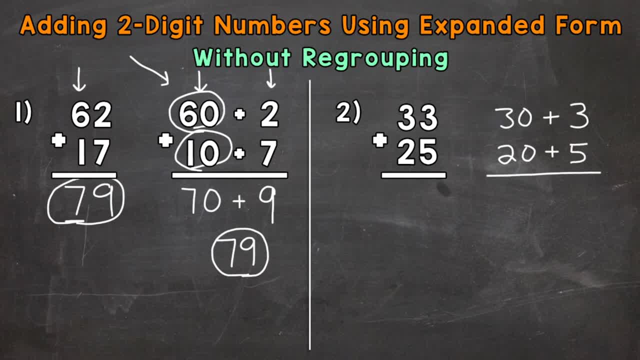 so notice our ones are lined up and our 10s are lined up. now we're ready to add. so we always start with our ones. three ones plus five ones gives us eight ones. bring down our addition sign and now we have 30 plus 20, which gives us 50.. let's add our ones and our tens and we get 58.. 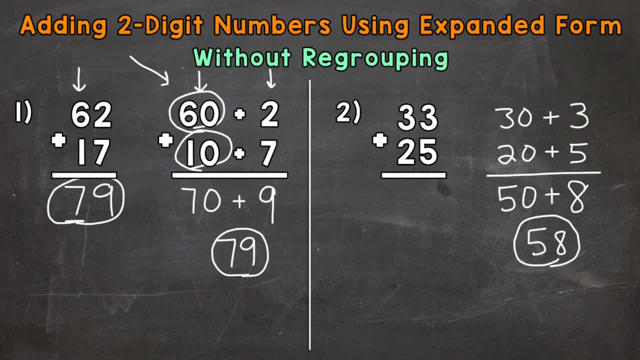 So our answer is 58.. Let's do the addition problem to the left and just add vertically, like we did for number 1, to see if we get the same thing. So 3 plus 5 in the ones place gives us 8.. 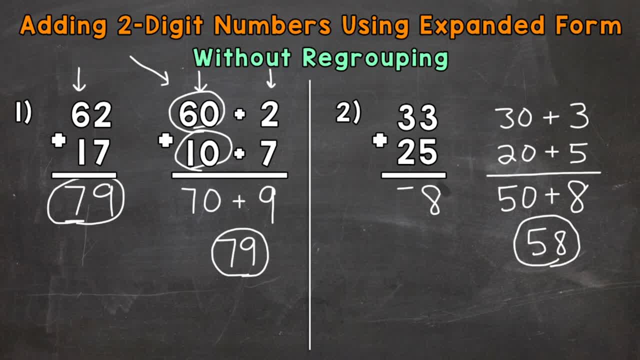 And 3 plus 2 in the tens place gives us 5., Which that's actually 50 because again it's in the tens place. Both ways we do this, we get 58. But again the expanded form. this is helping give us a deeper and better understanding of addition and what's actually happening within our addition problems. 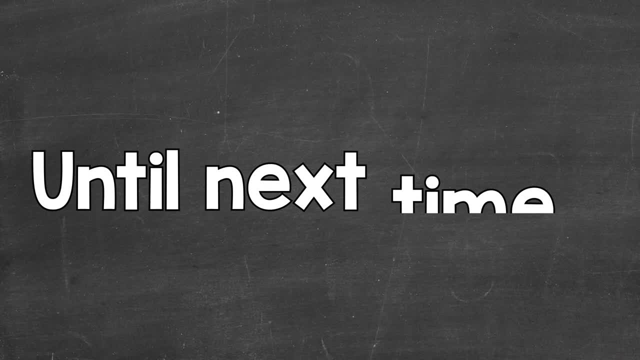 So I hope that helped. Thanks so much for watching. Until next time, Peace.